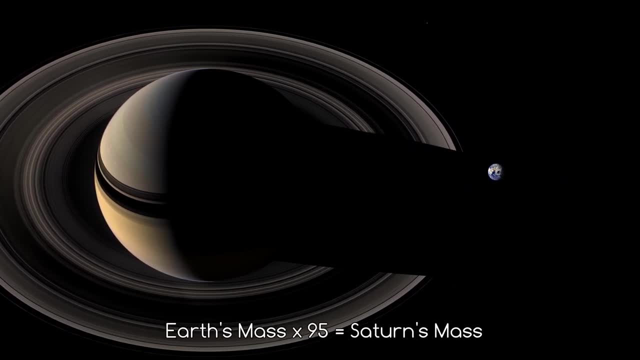 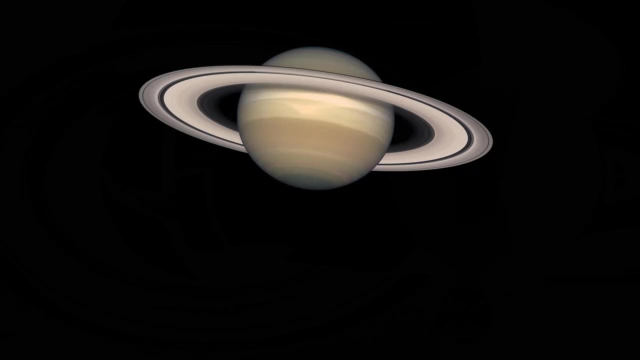 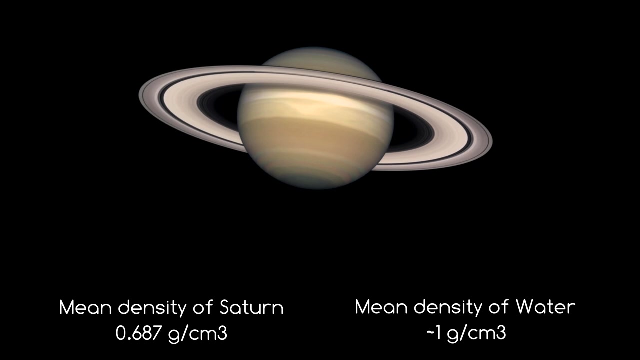 is so large. Saturn's mass is over 95 Earths. This low density makes Saturn the lightest planet per cm3 by far, and it's the only planet of the solar system that is less dense than water- about 30% less. so if you had a bath toy of Saturn that shares the same. 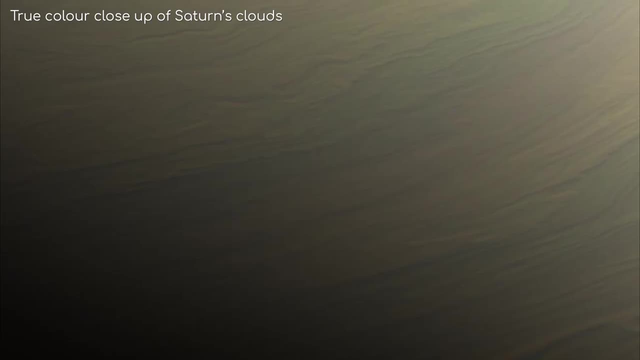 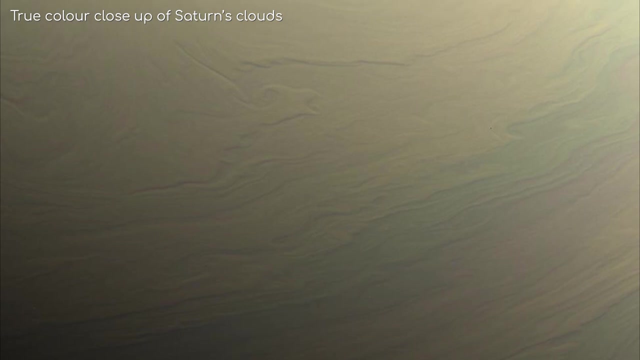 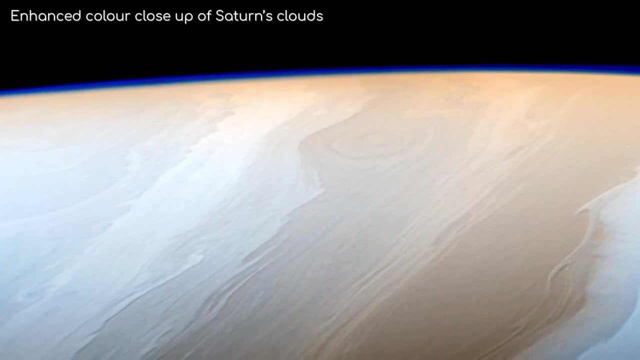 density as the planet it would float. This is because Saturn is 96% hydrogen, which is the lightest of the elements. However, average density doesn't tell the full picture of what a planet is like. Saturn is classified as a gas giant because what we see of the planet is simply gas. it doesn't. 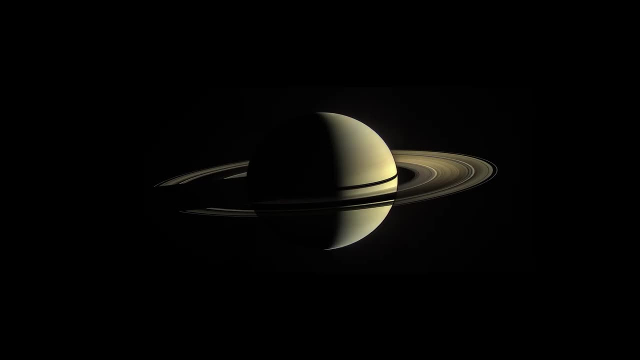 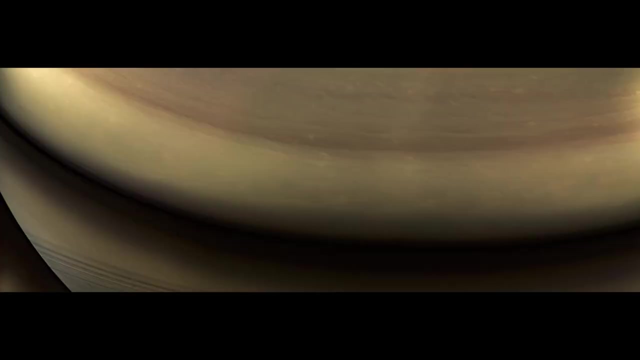 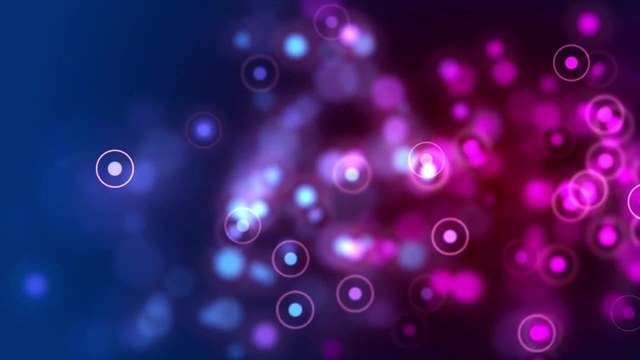 have a rocky surface under the cloud layer. However, Saturn is most certainly not gaseous all the way through. it's got too much mass for that. You see. the further into Saturn you go, the higher the pressure builds. Eventually the pressure becomes so great that the hydrogen 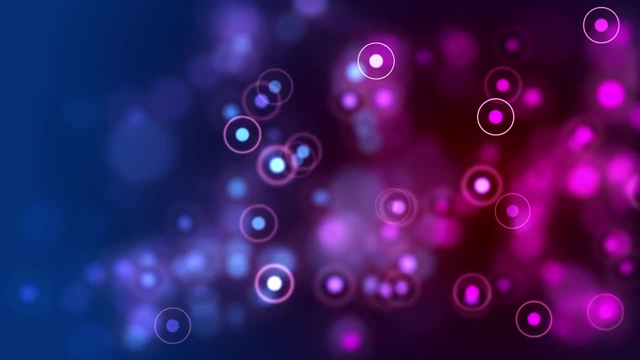 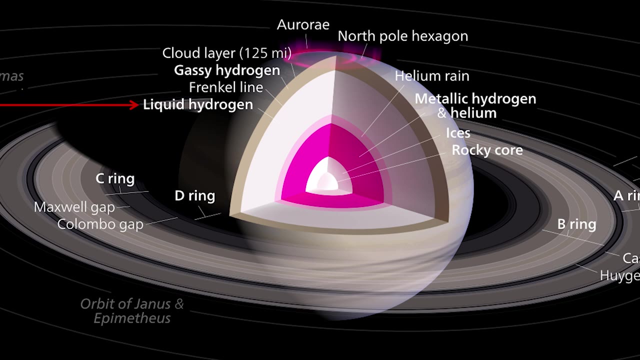 stops behaving like a gas and starts acting like a liquid. So, in a way, under Saturn's atmosphere is a liquid hydrogen ocean. Even further below that, it may be that there is a metallic hydrogen layer where the pressure is so great that hydrogen starts acting like 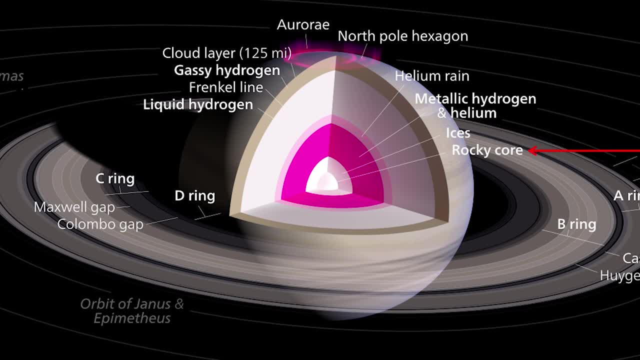 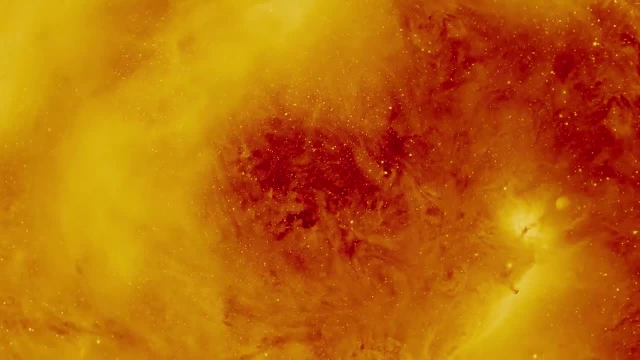 a metal and beneath that could be a metallic and rocky core. We do know that Saturn has a very hot interior, reaching 11.2 °C- 13.7 °C- 3.5 °C- 3.8 °C- 3.9 °C- 3.9 °C- 4.9 °C- 5.6 °C- 5.8 °C- 5.6 °C- 6.7 °C. 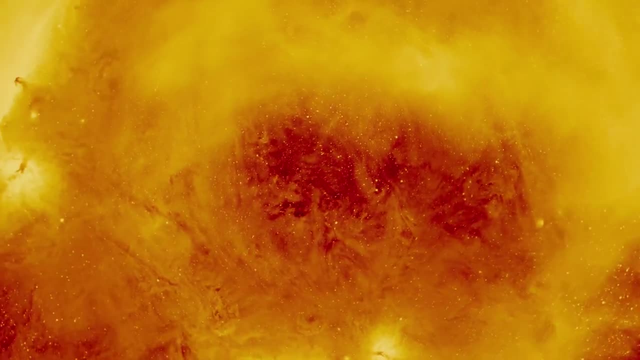 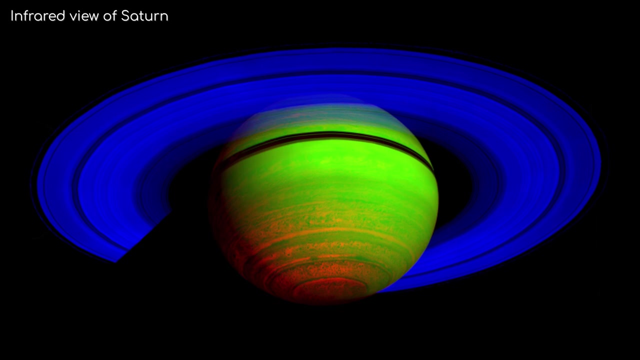 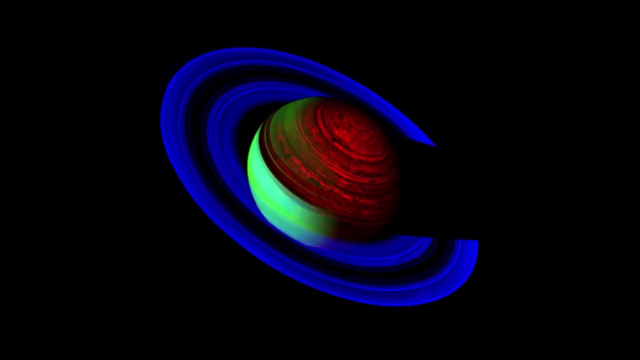 7,700°C at the core. This is twice as hot as the surface of the Sun. If we look at Saturn through the infrared, we can see Saturn's glow represented in brilliant shades of electric blue, sapphire and mint green. On the night side, where there 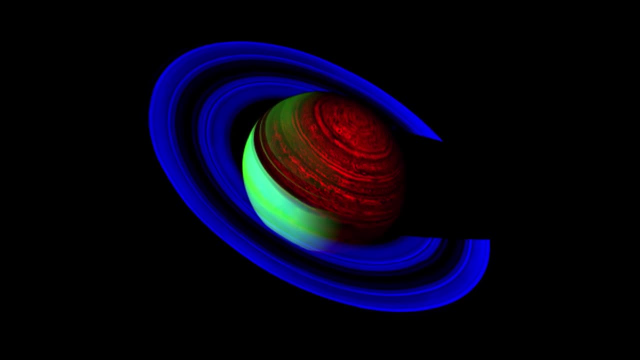 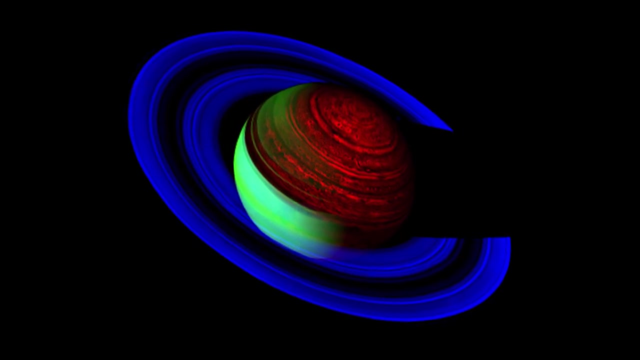 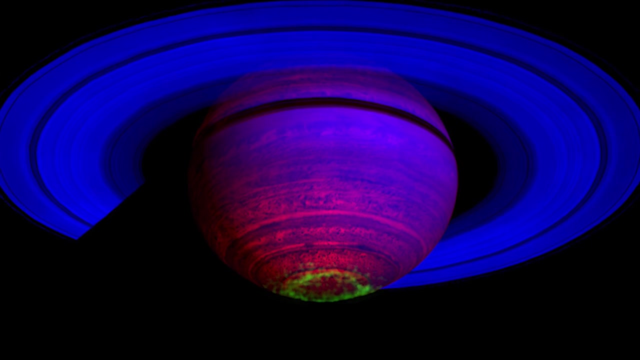 is no sunlight, Saturn's own thermal radiation lights things up. This light is generated deep within Saturn and it works its way upward, eventually escaping into space. In fact, this infrared image reveals that Saturn radiates 2.5 times more energy into space than it receives. 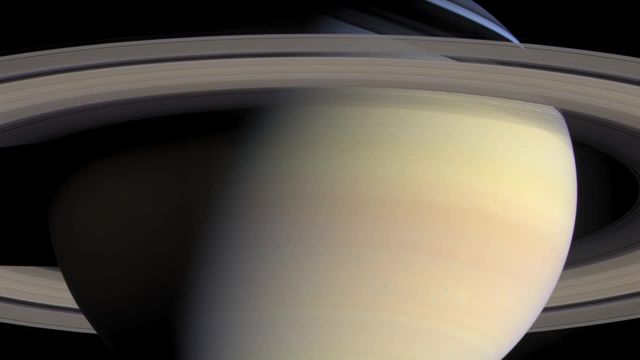 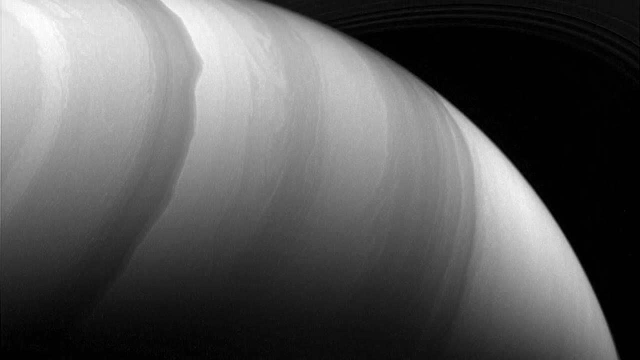 from the Sun. You may not have noticed, but Saturn's atmosphere has a banded pattern similar to Jupiter's. If you increase the contrast when you look at images of Saturn, this becomes more apparent. Saturn's bands are much less chaotic than Jupiter's, however. 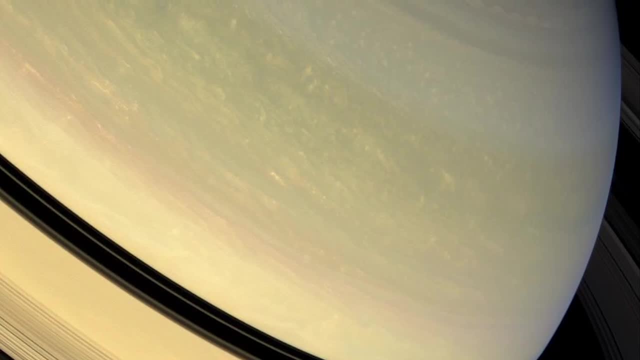 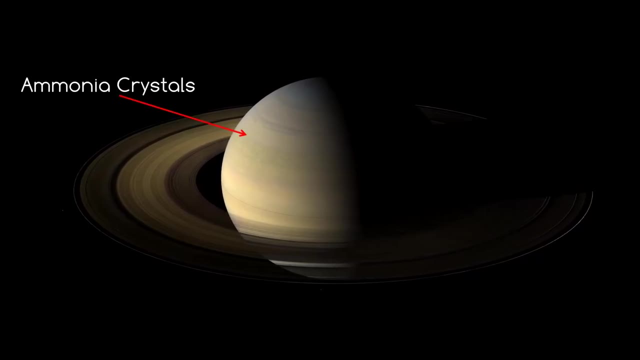 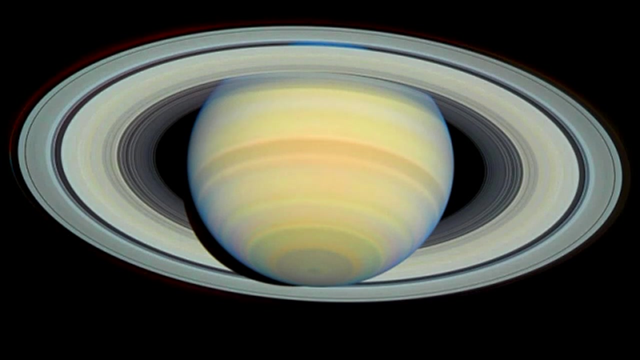 and are much wider near the equator, And ever wondered why Saturn is yellow? It's believed to be due to ammonia crystals in the upper atmosphere. But while the atmosphere of Saturn may appear calm, the planet is actually extremely active. The winds on Saturn are the second fastest among the solar system's. 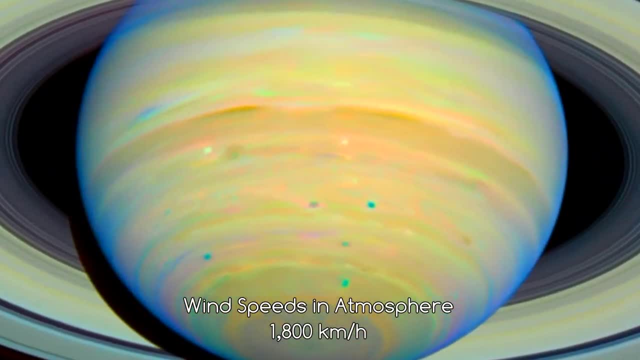 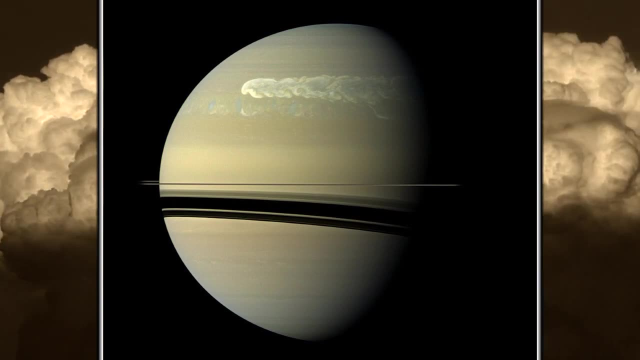 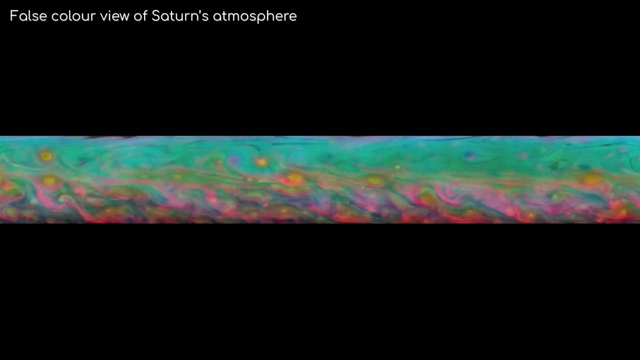 planets after Neptune, They can be a blistering 1,800 km per hour. Visible storms are also known to appear on Saturn, like this one that lasted just under a year in 2011.. It had been the pattern that every 30 or so Earth years, the planet produces what is called 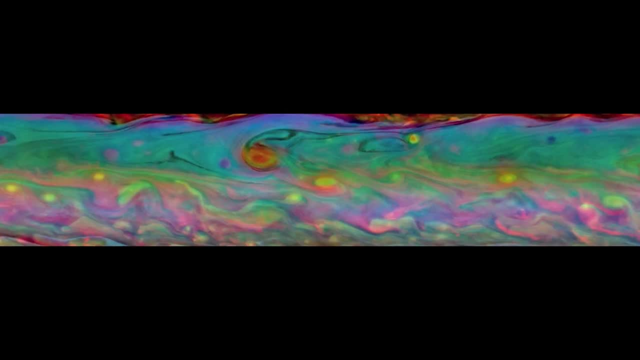 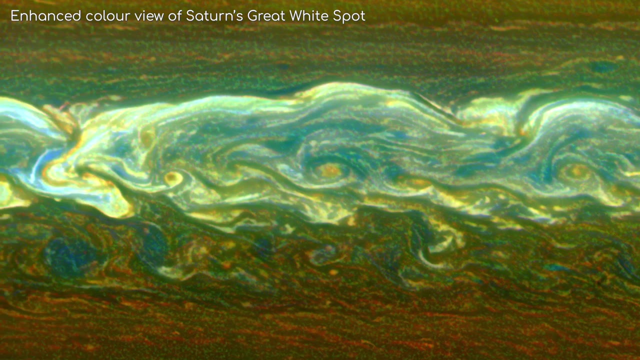 a great white spot, which is a unique but short-lived phenomenon, believed to occur once every Saturnian year. However, we have spotted a few of them over the last 30 years. If it does follow a 30-year pattern, though, we can expect another one any time now. 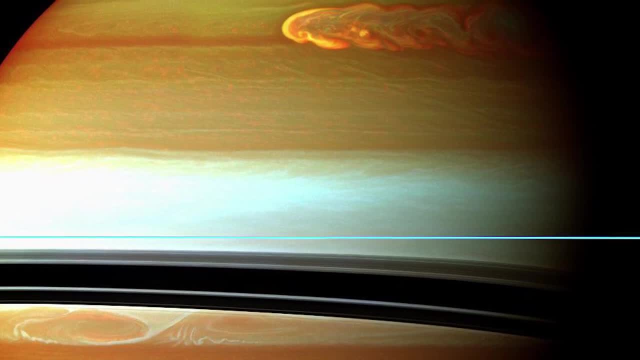 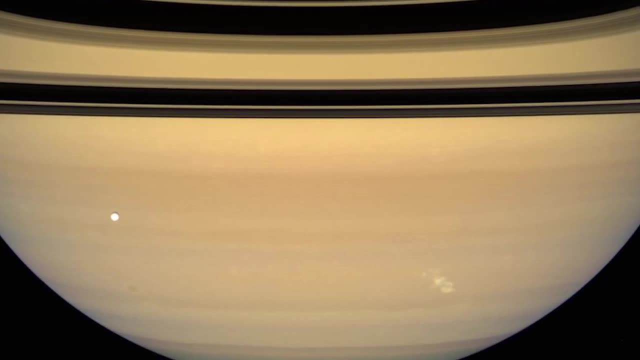 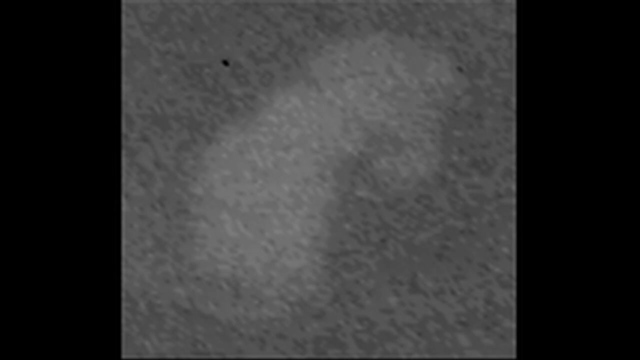 Sadly, even if it does happen, we will only be able to see it through the Hubble Space Telescope, as the Cassini mission ended a few years back. Saturn has plenty of smaller storms too, where lightning is often produced. Cassini has even detected the sound of thunder. 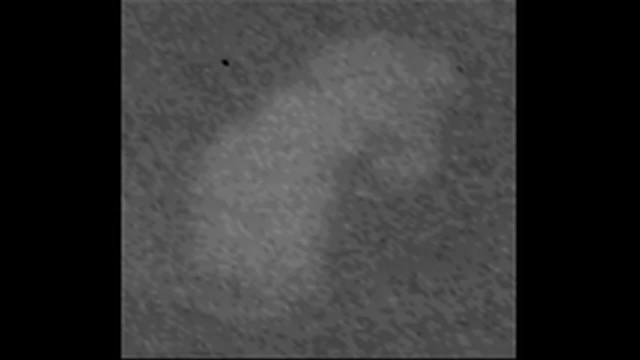 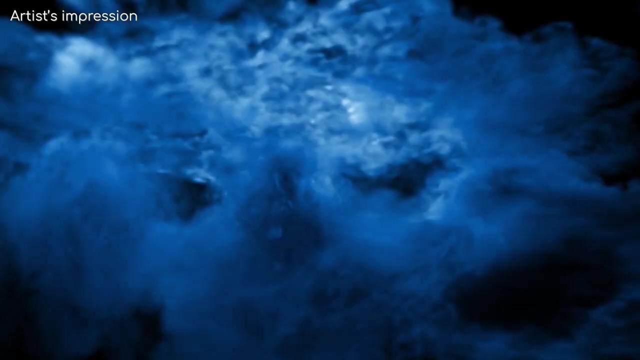 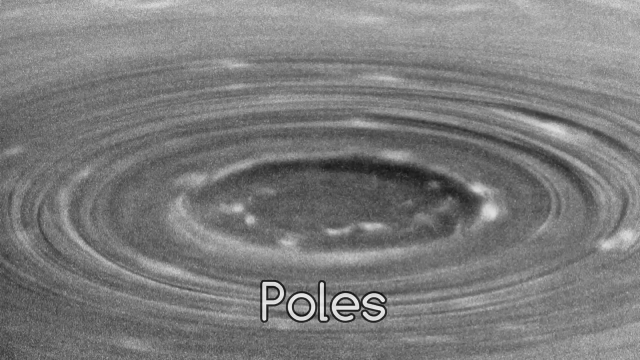 While this might sound weak, the sound you are hearing is actually the radio waves produced by the lightning. In reality, lightning on Saturn is about 1,000 times more powerful than what we see on Earth. Still talking about storms, but moving on to the planet's poles, we find that each 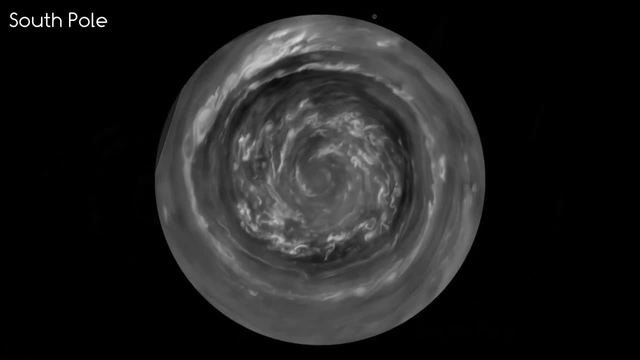 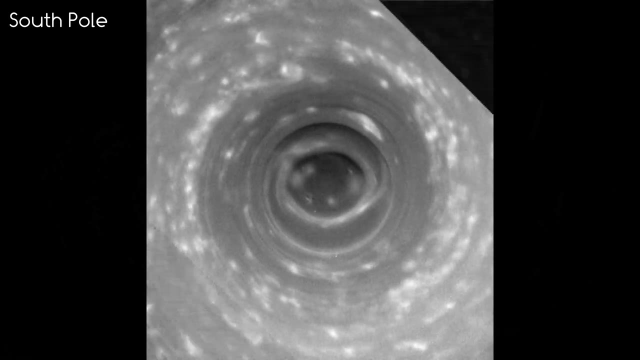 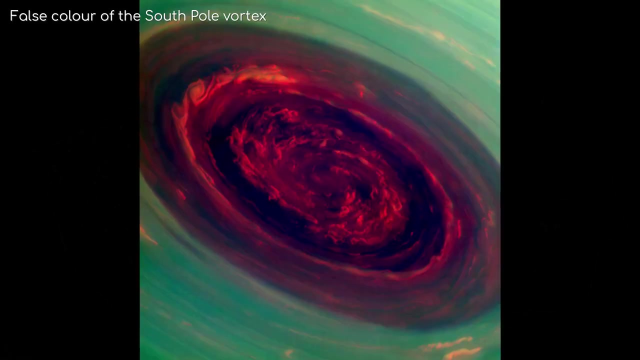 pole has giant permanent storms. NASA reported in November 2006 that Cassini had observed a hurricane-like storm locked to the south pole that had a clearly defined eyewall. Eyewall had not previously been seen on any planet other than Earth. The ring is similar to the. 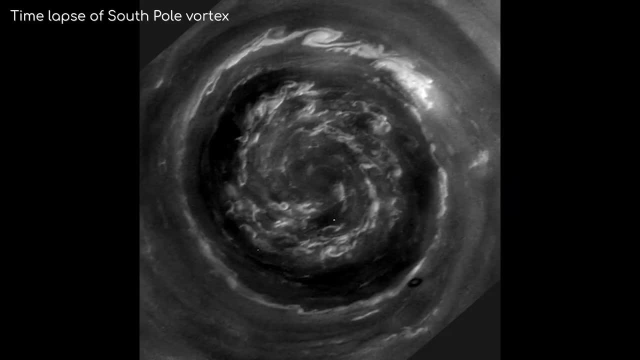 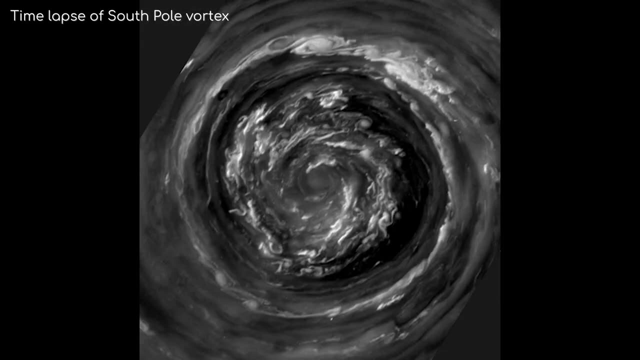 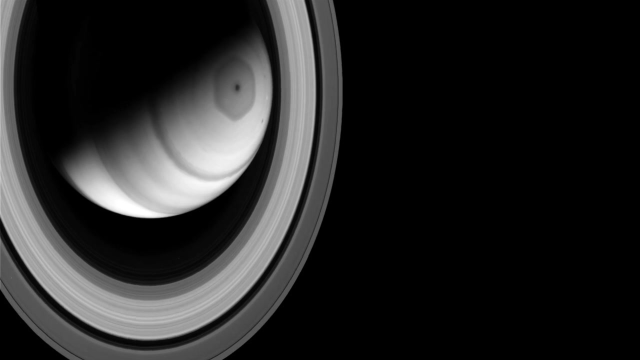 eyewall of a hurricane, but much larger. The clear air in the centre is warm like the eye of a hurricane, but on Saturn it is locked to the pole, whereas a hurricane on Earth drifts around. The North Pole is even more unusual. There is a persistent hexagon-shaped storm that rotates with the planet, not with the atmosphere. However, the gravitational pull of the hurricane is less powerful than those of Mars, and the Expressway is much more powerful than those of Mars. All the more reason to keep watching and see these videos. 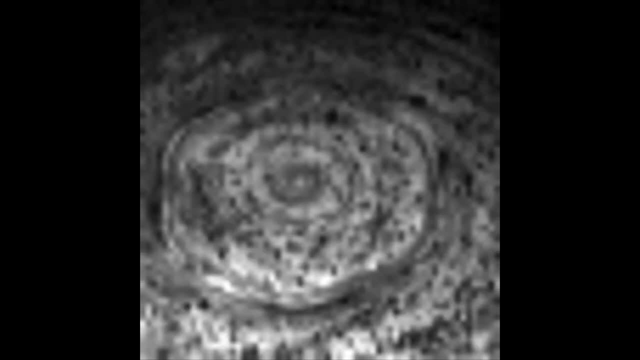 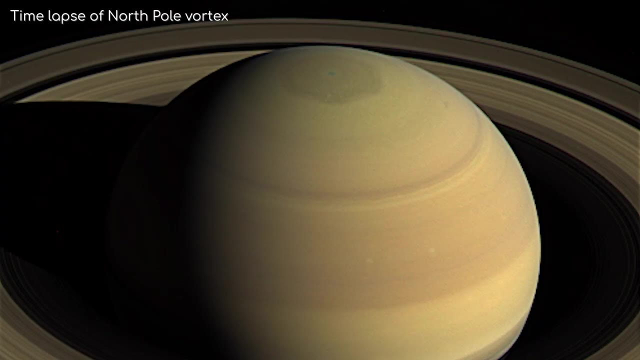 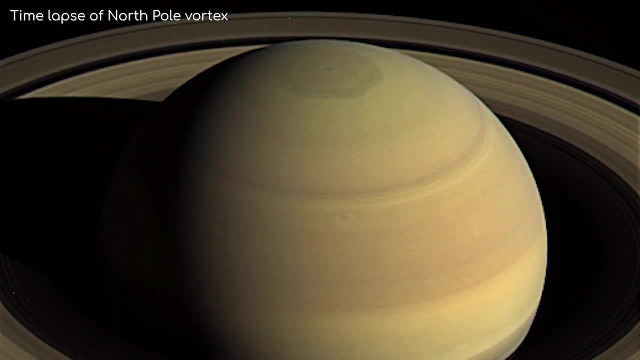 The straight sides of the polar hexagon are each about 13,800km long, making them larger than the diameter of the Earth. Why does this happen, and to such a large scale? Well, we don't really know, However, the speed differential and the viscosity parameters between atmospheric bands here 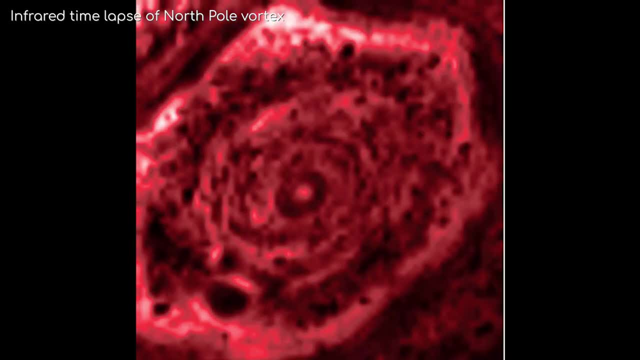 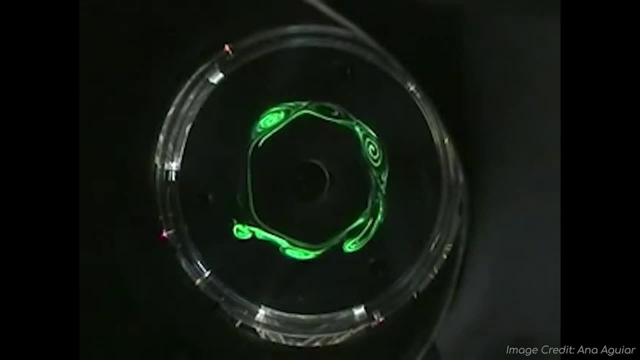 are likely to be within certain margins to allow such an unusual polygon to form. Lab tests have since been done where polygons could form in a circular tank of liquid, rotated at different speeds at its centre and near the outer boundary. so this is the leading. 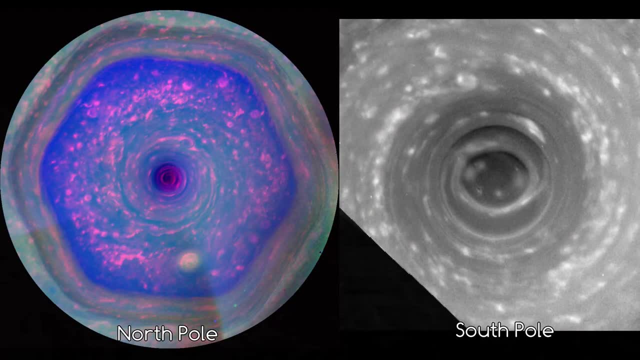 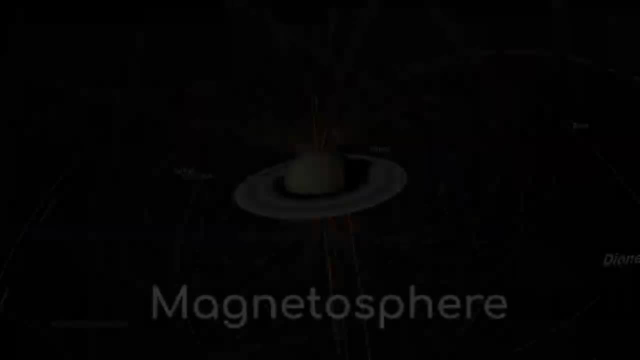 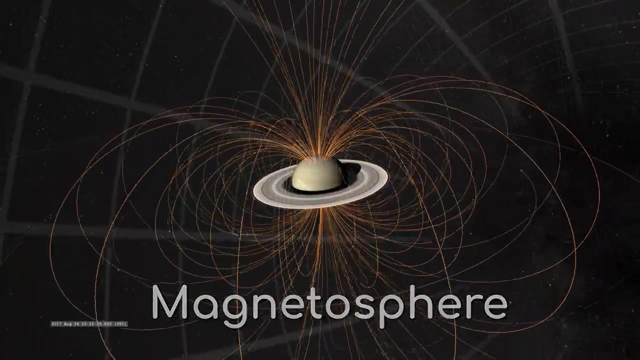 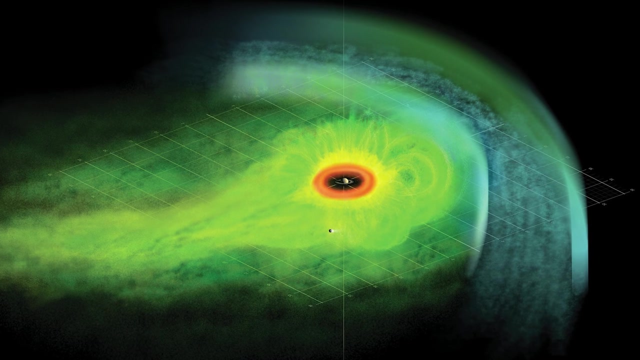 theory at the moment. Interestingly, towards the centre of this hexagon, another eye wall can be found. While not anywhere near as strong as Jupiter's, Saturn does have a magnetosphere potentially generated in the metallic hydrogen layer of the planet. It is large, extending far beyond the planet, and it is strong enough to deflect solar wind. 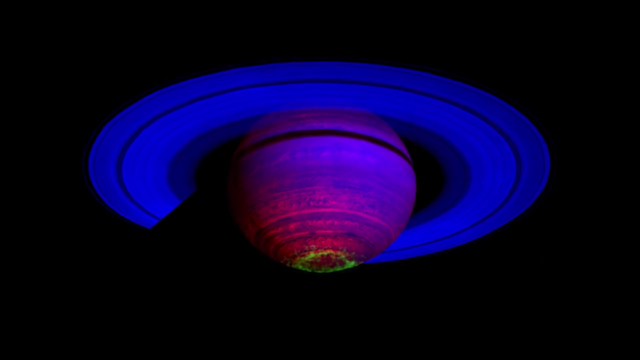 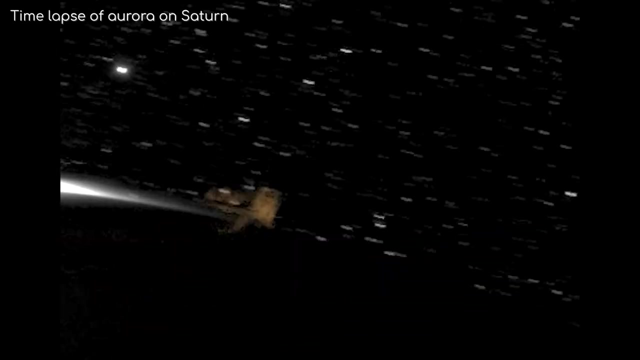 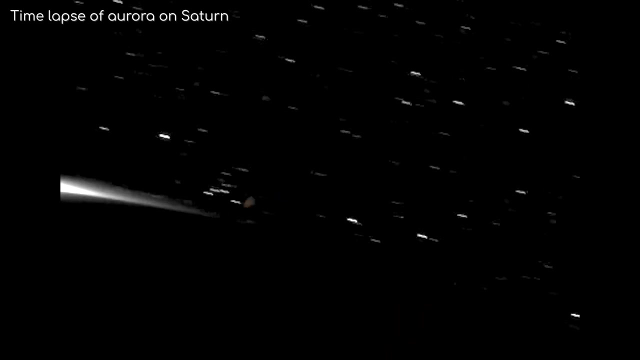 from the Sun And much like other planets with magnetospheres, Saturn has auroras. Their location and brightness strongly depend on the solar wind pressure. The auroras become brighter and move closer to the poles when the solar wind pressure increases. The same process produces auroras on both Earth and Saturn, where electrons from the 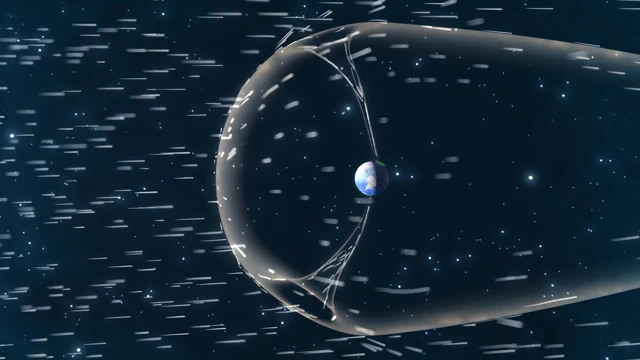 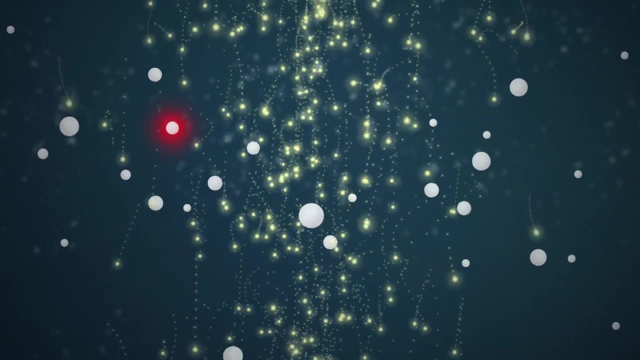 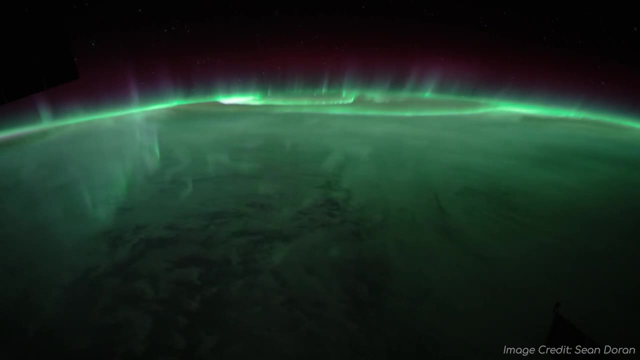 solar wind stream along the magnetic field lines, directed into the upper atmosphere. There they collide with atoms and molecules, exciting them to higher energies. The atoms and molecules release this added energy by radiating light at different colours and wavelengths. On Earth, this light is mostly from oxygen atoms and nitrogen molecules. 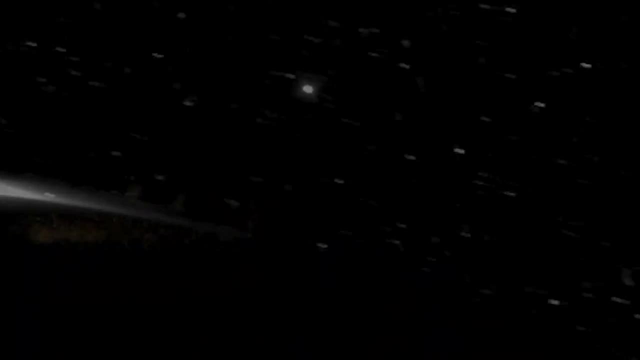 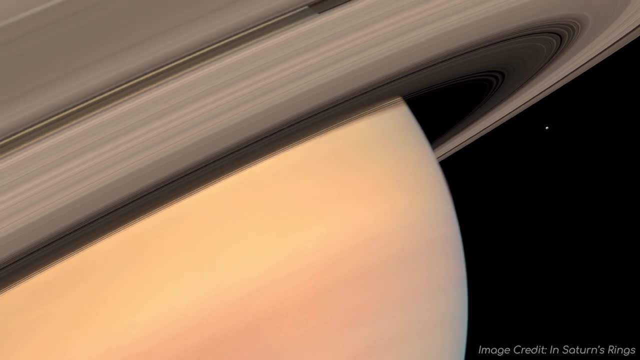 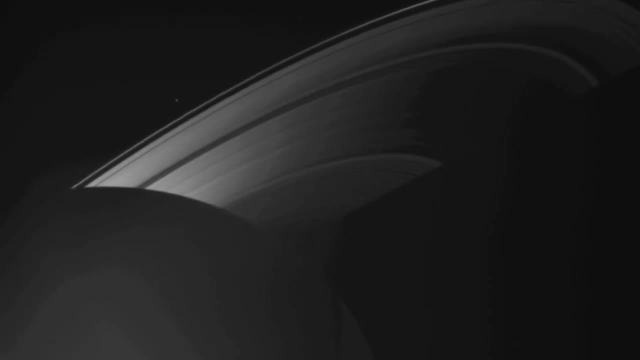 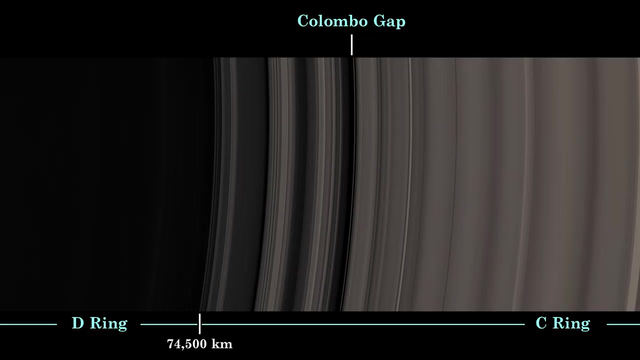 Saturn has a prominent ring system that consists of 10 continuous main rings. While they are mainly named after letters of the alphabet, the naming conventions are a little confusing, so bear with me. The first five rings, from the closest to the planet outward, are the D-ring, which 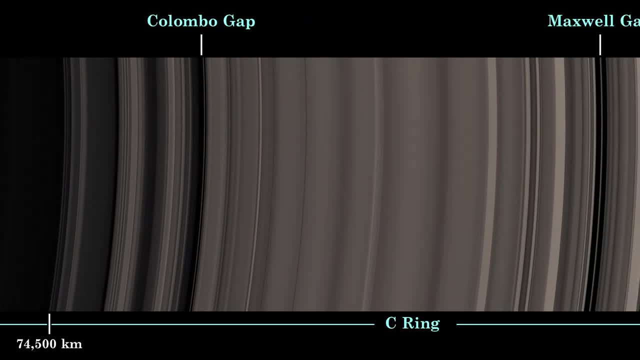 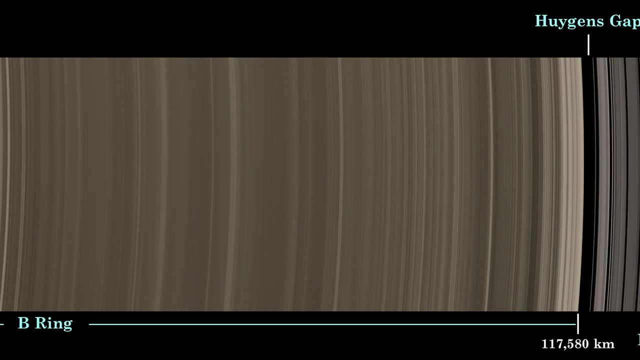 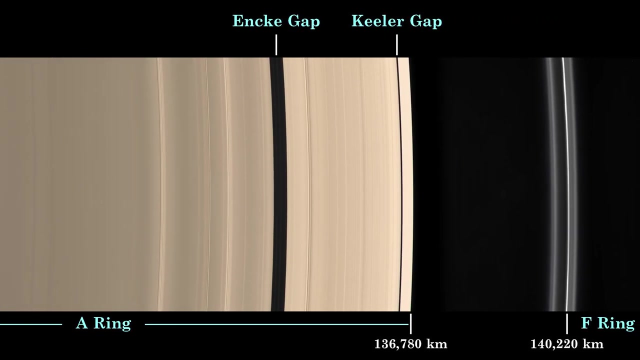 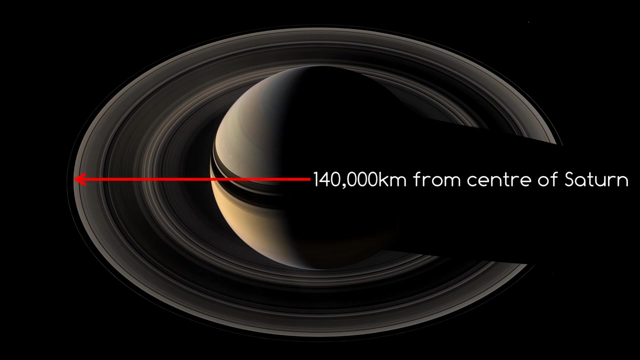 is very faint: the C-ring, B-ring, which is the brightest and widest of all the rings, the A-ring, which is the last of the large bright rings, and then the F-ring. The rings extend from 66,000km to 140,000km above Saturn's centre and are made up mostly: 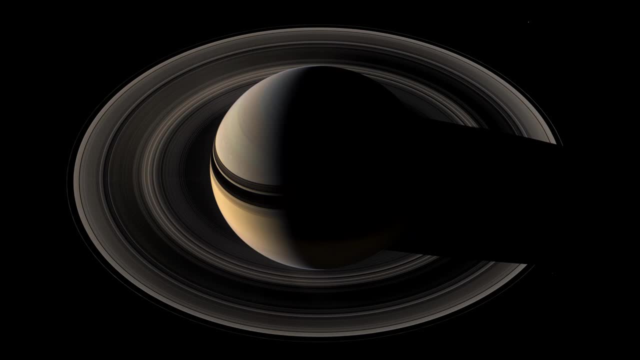 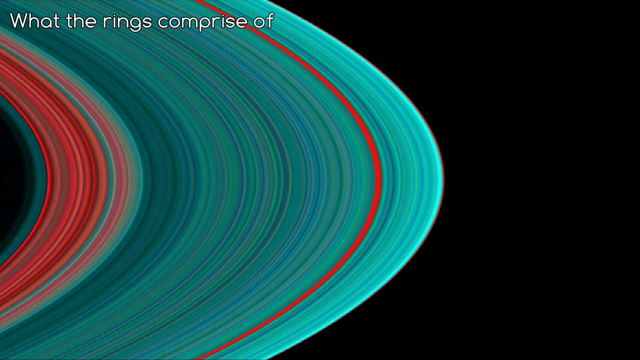 of water, ice, with small amounts of dust and rocks. If we look in the ultraviolet at a section of the brightest rings, it shows there is more ice towards the outer part of the rings than in the inner part. The red in the image indicates sparser ringlets, likely made of dirty and possibly smaller. 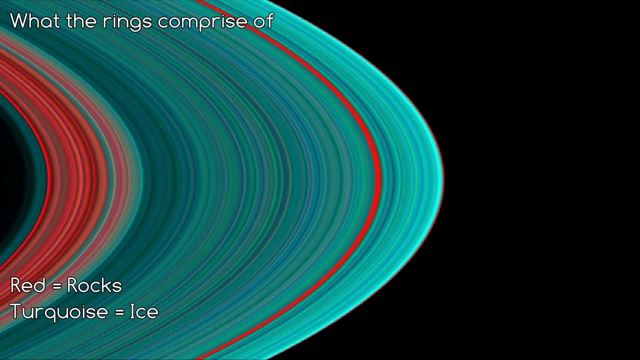 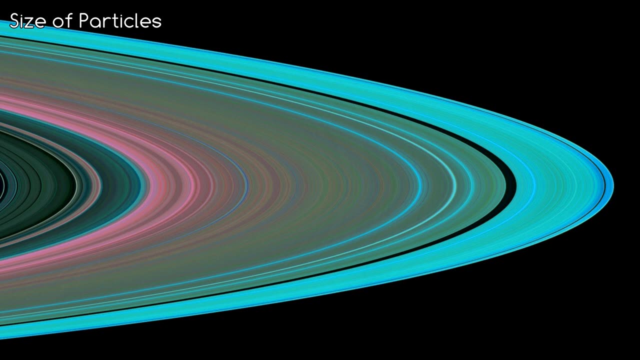 particles than in the icier turquoise ringlets. If we look at a picture representing radio occultation, we can judge the size of the individual particles that make up the rings. Colour is used to represent information about ring particle sizes based on the measured effects of three radio signals. 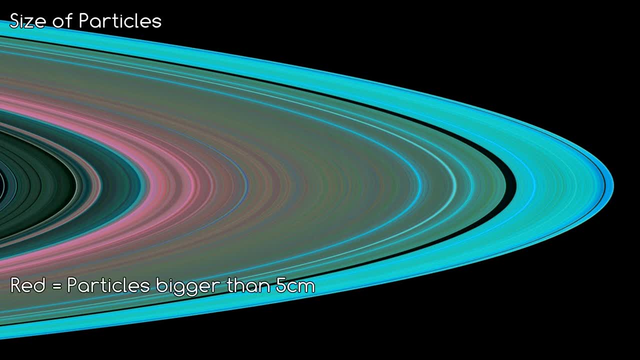 Shades of red show regions where particles are larger than 5cm in diameter, Green shows particles smaller than 5cm and blues show particles less than 1cm in size. Overall, it's thought that particles in the rings aren't bigger than 10m, and most 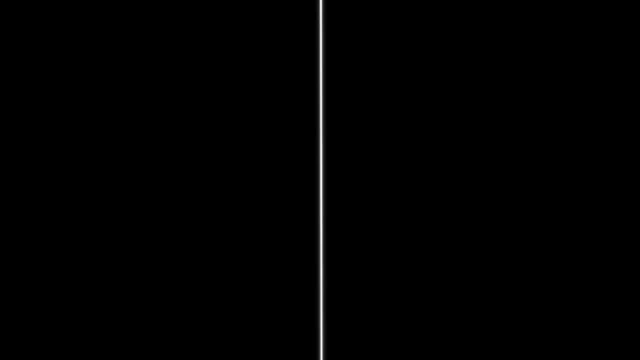 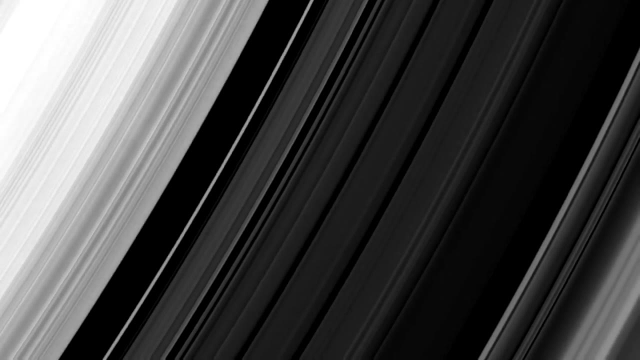 are microscopic in size. The main rings are thought to be as little as 10m thick to 1km thick. We can see that the rings are not perfectly symmetrical. During the planet's equinox, the rings can get a bit wonky. 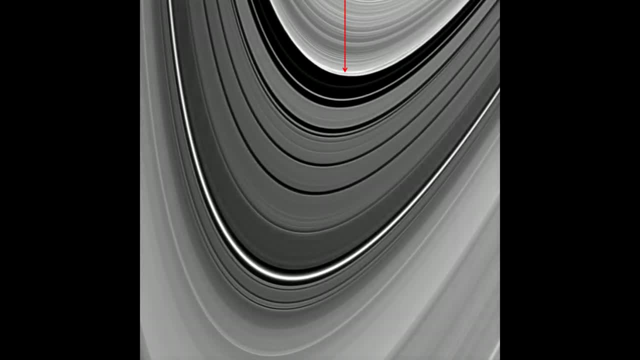 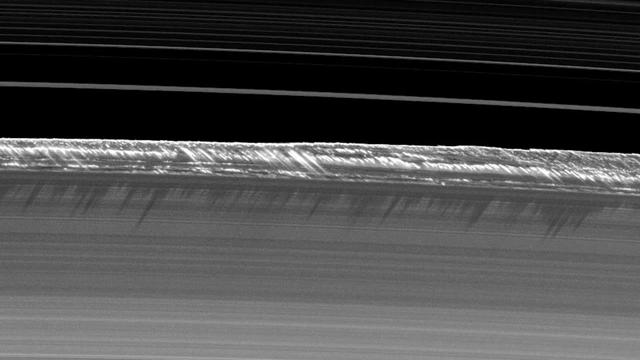 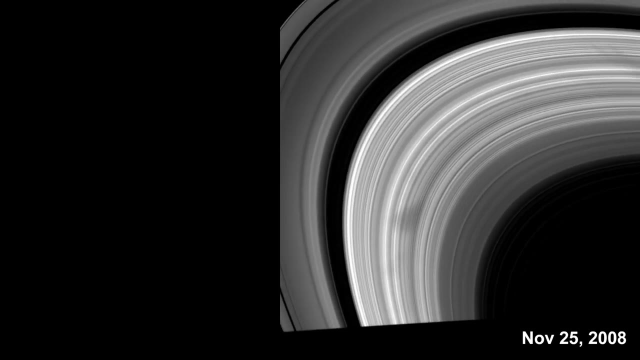 Look at the top of this video where the B ring meets the A ring. Zooming in on this structure reveals ridges and spokes a couple of kilometres tall, their presence given away by their shadows. Zooming out again, we can see the scale of how many spokes there are during this period. 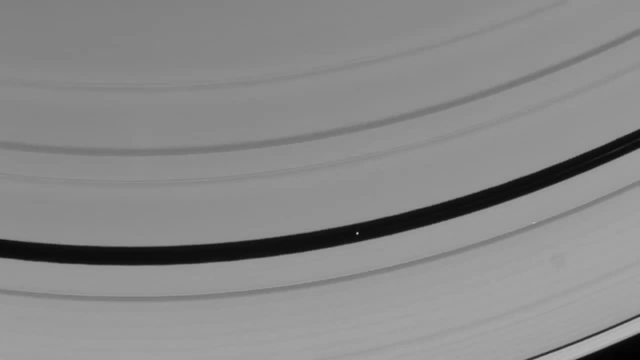 Oscillations happen all the time in the rings, though, perhaps due to the presence of a shepherd moon or even just naturally. The difference is we don't see them all the time in the rings. The difference is we don't see them all the time in the rings. 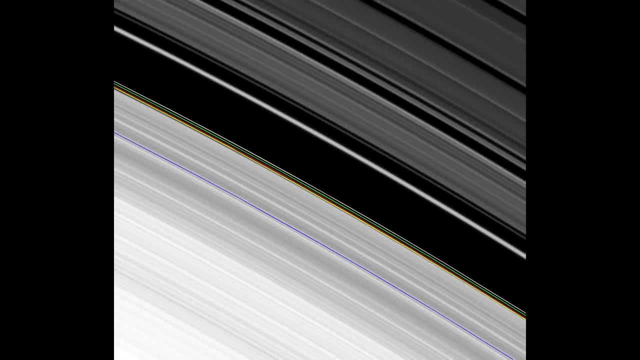 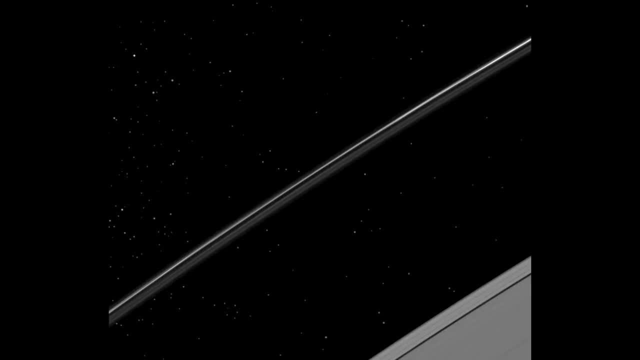 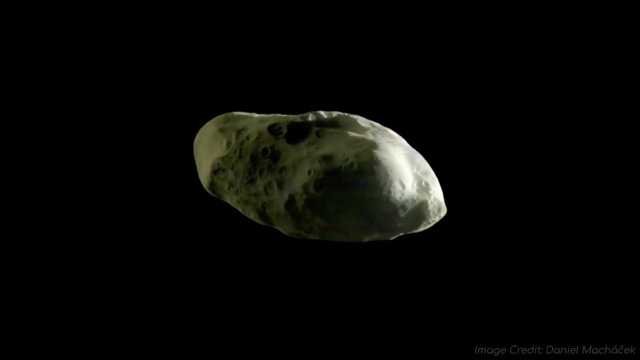 Most of the rings which can be seen all in only a day can be up to 200km. So I've talked about the D, C, B and A rings and also mentioned the F ring. The F ring can also get quite wonky and has a perfect example of what is called a shepherd. 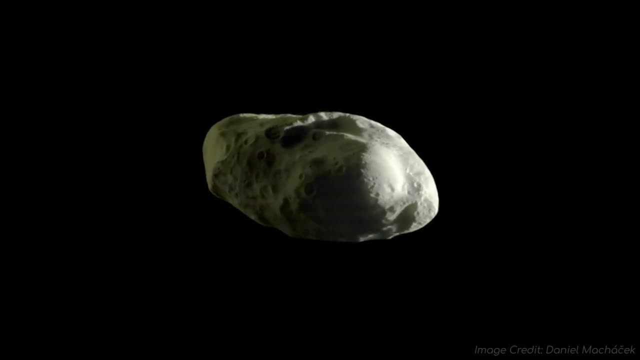 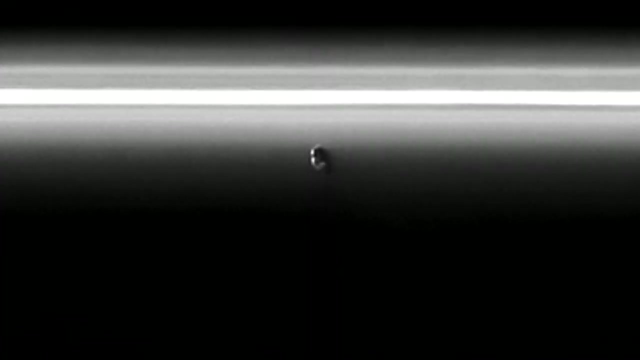 moon. It's called Prometheus and it leaves a beautiful ripple in the F ring as it orbits. Once during its 14.7 hour orbit of Saturn Prometheus, which is only one hundred and two seconds later, it's still going up and it's a bit sweltering. 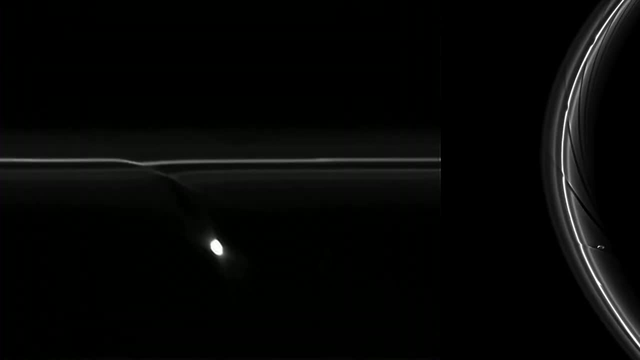 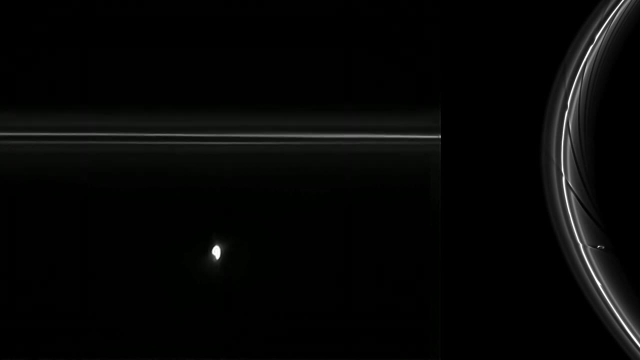 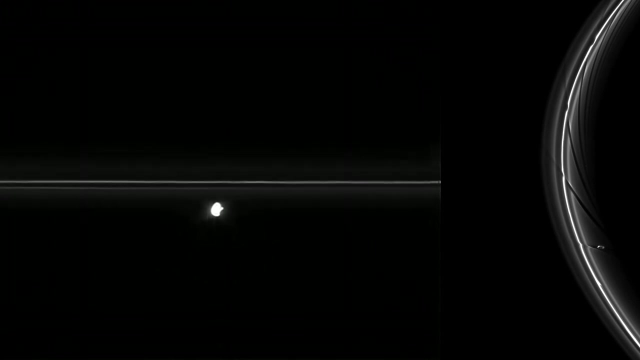 102km across, reaches the point in its elliptical path where it is farthest away from Saturn and closest to the F ring. At this point, Prometheus' gravity is just strong enough to draw a streamer of material out of the core region of the F ring, and that's what causes these ripples. 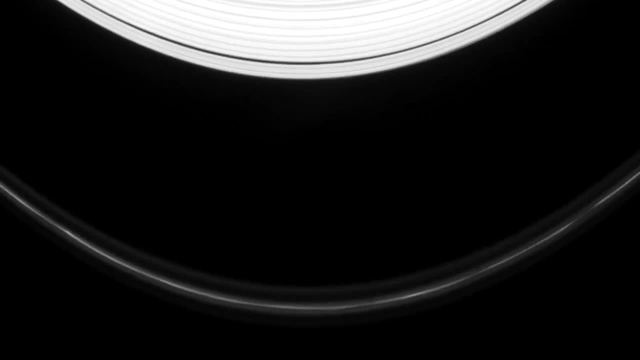 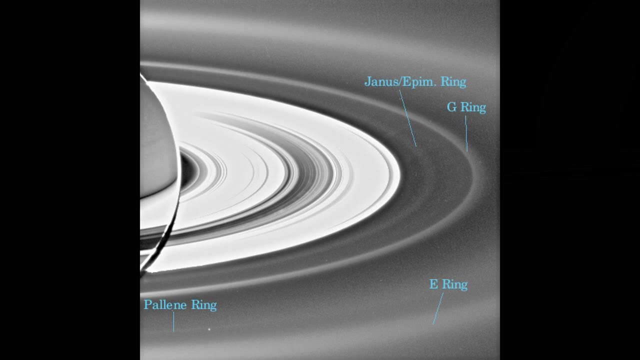 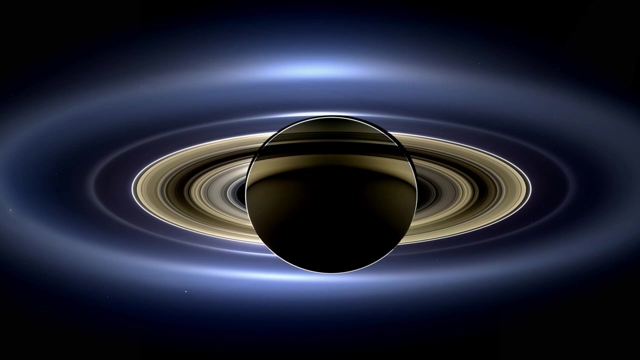 So what comes after the F ring? Well, this is where it gets confusing. First you have the Janus or Epimetheus ring, The G ring, Pelleni ring and then the E ring. I find this picture amazing, as these rings are much more visible, being backlit by the 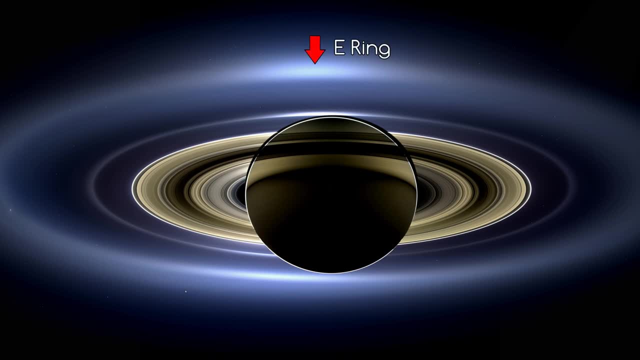 Sun. This bright blue ring is the E ring and you can just about see the faint Pelleni ring at the top of this picture. The G ring is the next distinct ring and again you can just about see the Janus or Epimetheus ring at the top below it. 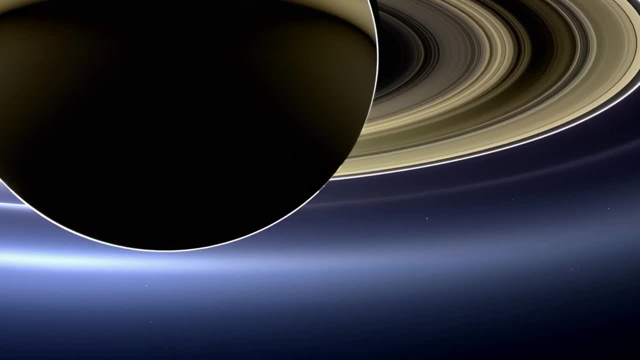 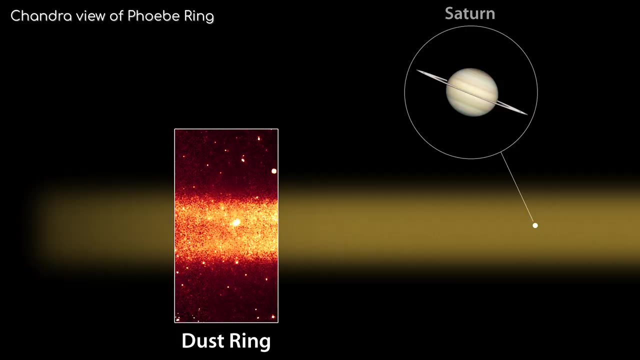 And can you see us? We are all in this picture. Here's Earth and the Moon. The very last ring is the newly discovered Phoebe ring, a huge yet dispersed ring that extends far beyond Saturn. It's so large that, if it were visible from Earth, its apparent diameter would be the. size of two full moons across. It probably originated from Saturn's 200km wide moon, Phoebe, which had been battered in its past. Phoebe orbits just outside of the ring and probably keeps this dust contained from going outward. On the other hand, it is also suspected that dust in this ring is falling inward eventually. 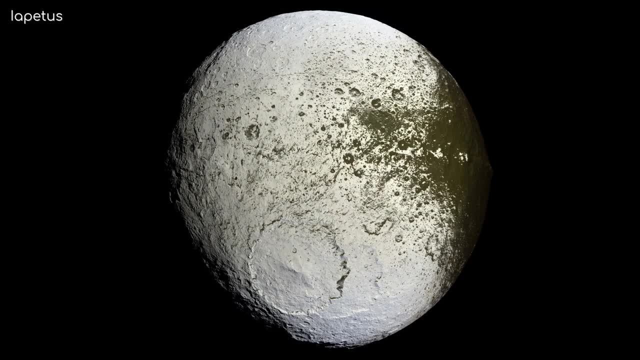 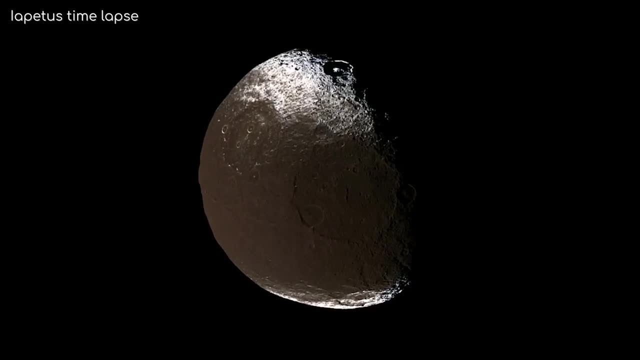 falling into Iapetus, Saturn's outermost regular moon. It has a bizarre combination of colours because dust from the Phoebe ring settles on it, But because Iapetus is tidally locked, only one side of the moon ever faces Saturn with. the Moon. This means that Saturn is the only side of the Moon that ever faces Saturn. This means that Saturn is the only side of the Moon that ever faces Saturn. This means that Saturn is the only side of the Moon that ever faces Saturn. 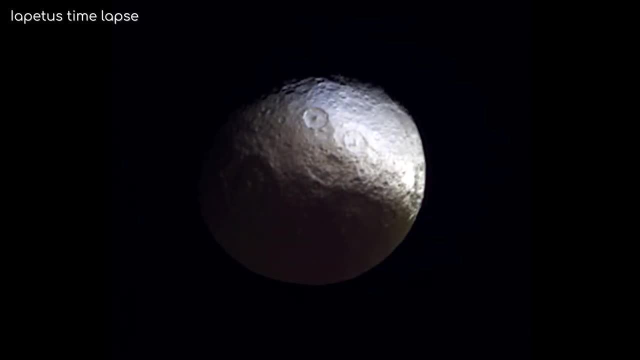 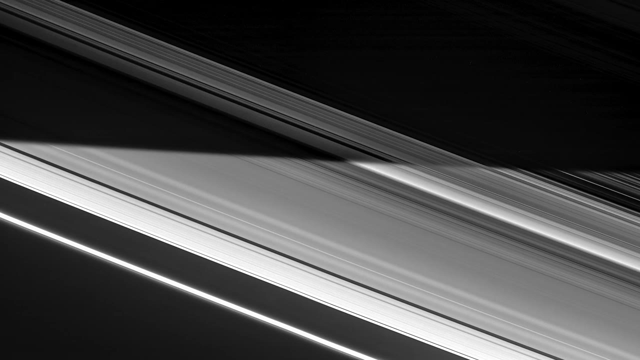 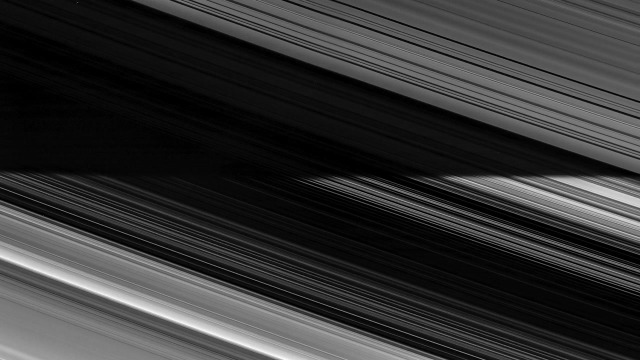 And it's the backside of it exposed to the Phoebe ring, meaning its two faces look very different. So now you know about the rings, I think you'll agree that they are so interesting in their own right. Theories abound as to why they are there, but we simply don't know. 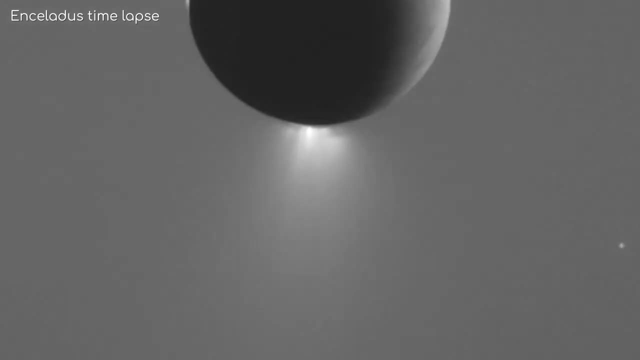 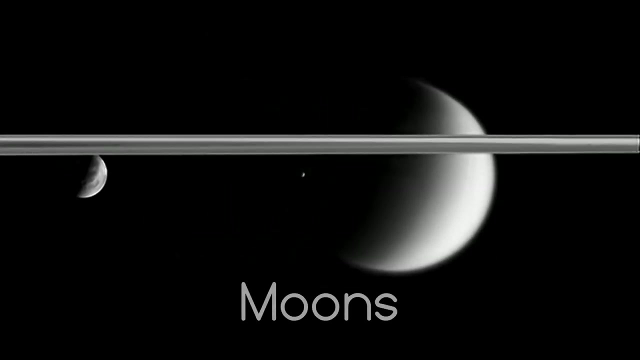 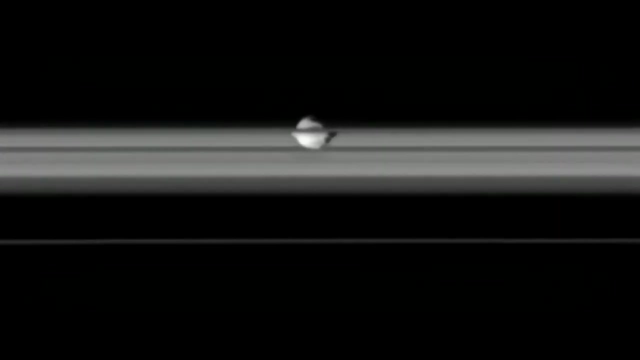 We know that some of the moons are responsible for some of the material there, and we also know that some of the material there is responsible for some of the moons. And talking of moons, Saturn has at least 82 of them. They come in all shapes and sizes and, most uniquely, Saturn's largest moon, Titan. 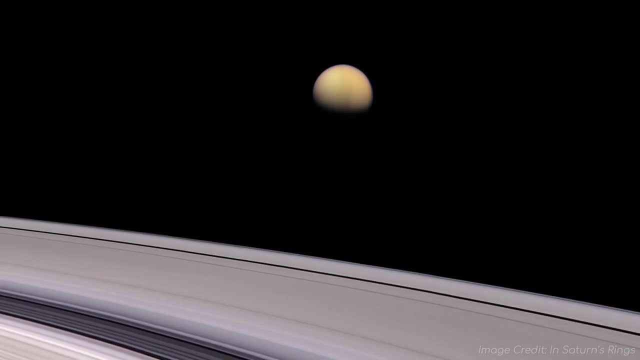 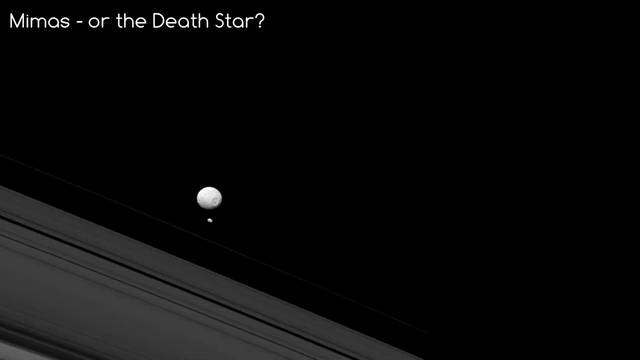 which is even bigger than Mercury, is the only moon in the solar system with a thick atmosphere around it, which I have done a separate video about here. I'm also going to throw in here that Saturn has the Death Star orbiting it, biding its. 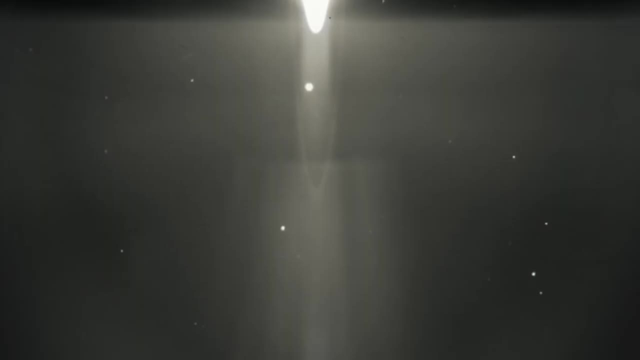 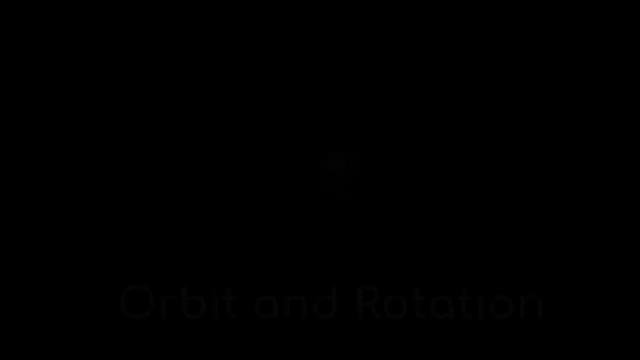 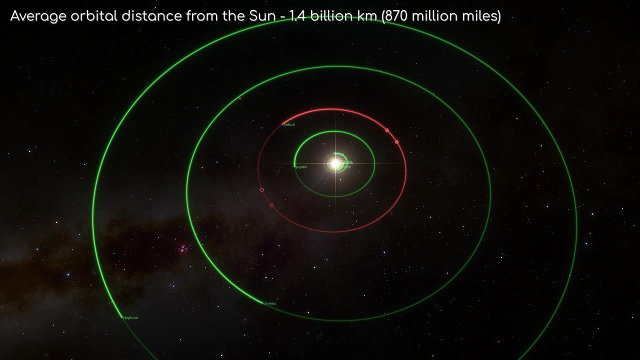 time We call it Mimas. Generally, though, Moons are very small, only a few kilometres across. Lastly, I'm going to talk about Saturn's orbit. Saturn orbits about 9-10 times further away from the Sun than Earth does, and one year. 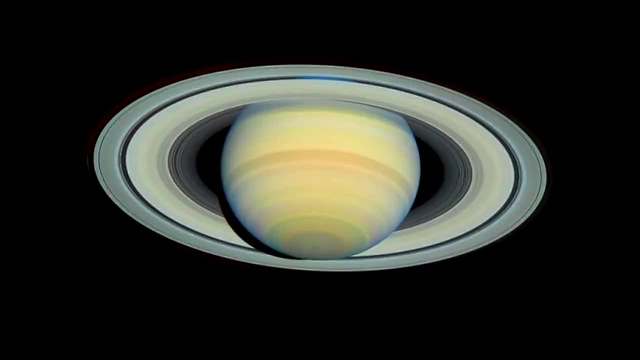 on Saturn takes 30 Earth years. Funnily enough, a day on Saturn is different depending on where you are situated: At the equator or at the poles, a day lasts about 10 hours and 14 minutes. Everywhere else on Saturn, a day lasts about 10 hours and 14 minutes. 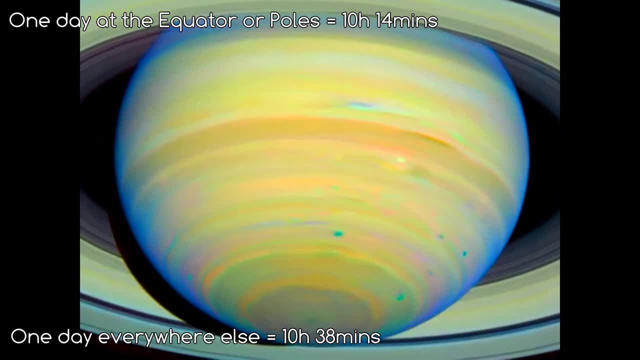 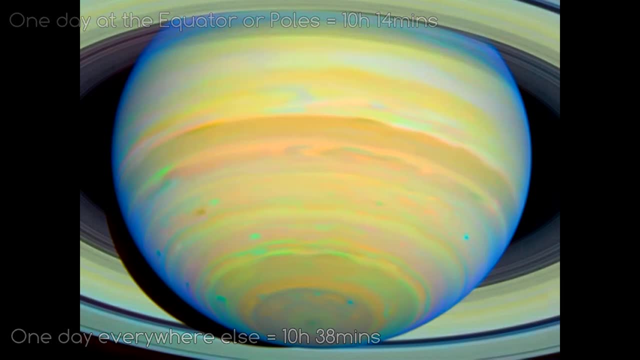 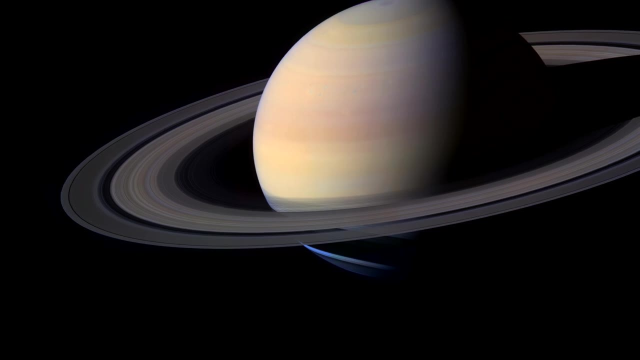 A day lasts about 10 hours and 38 minutes. The issue is: because Saturn isn't solid, it's not bound to rotate at the same speed all over. I just want to leave you with this: Few sights in the solar system are more strikingly beautiful than softly hued Saturn embraced. 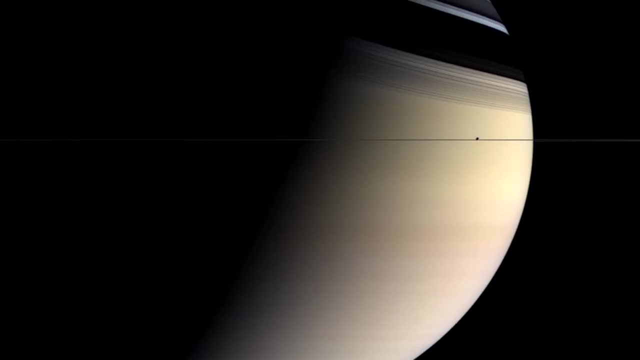 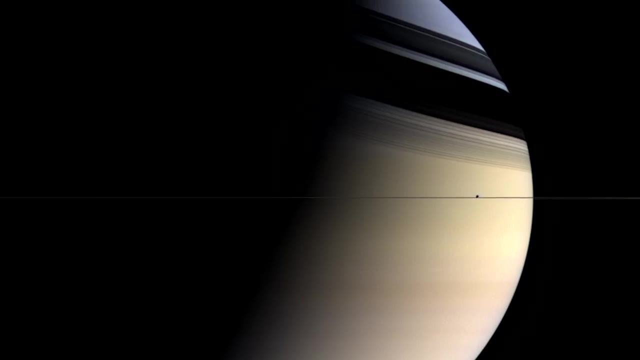 by the shadow of its rings. The gas planet's subtle northward gradation from gold to azure is a striking visual effect that scientists don't fully understand. The gas planet's subtle northward gradation from gold to azure is a striking visual effect that scientists don't fully understand.